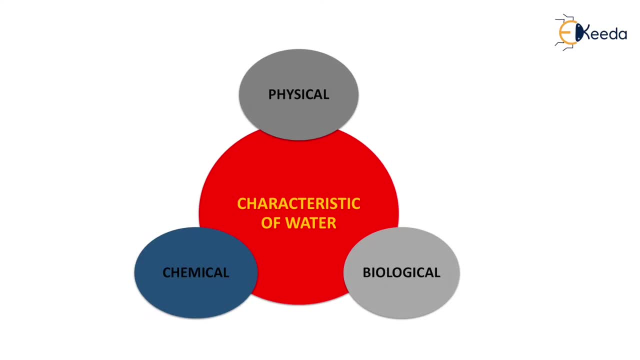 then that water is fit for drinking purpose. otherwise that water needs treatment. That's why we are going to study the characteristic of water Now. we had divided the characteristic of water into three parts, that is, the physical characteristic, the chemical characteristic and the biological characteristic. 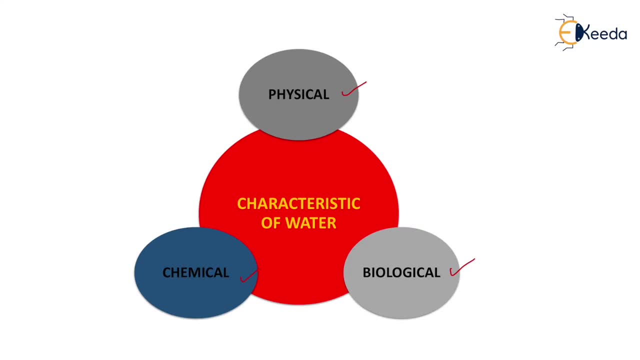 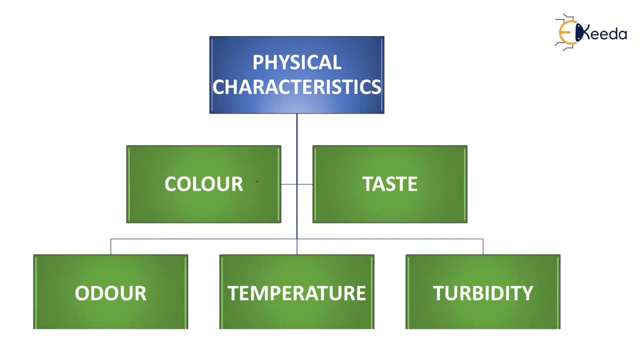 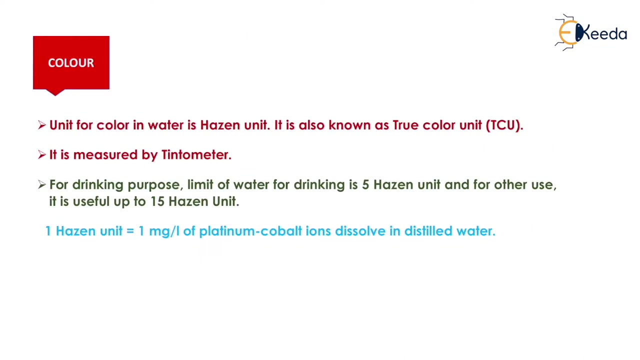 We will see each and every parameter in detail, one by one, starting with the physical characteristic. Now we had subdivided the physical characteristic into the following types, that is, color, taste, odor, temperature and turbidity. Now, starting with the color, 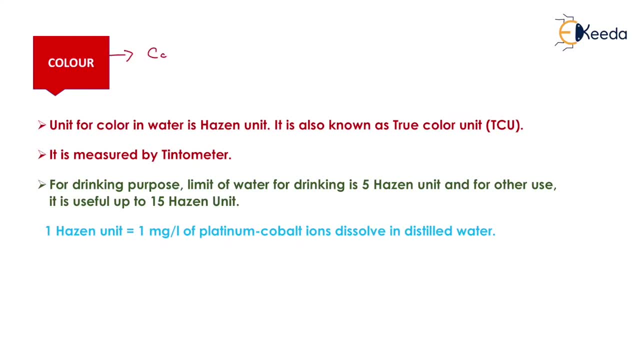 what is the color of drinking water? Generally, the color of drinking water will be colorless. Now, if we want to measure the color, in which unit we are going to measure the color? Generally, the color is measured in hazen unit. 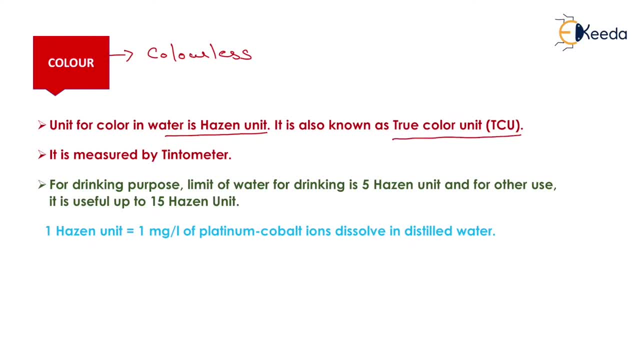 or it is equivalent to true color unit. Now the question arises that what is one hazen? It will be equal to one milligram of platinum cobalt ion dissolved in one liter of distilled water. It means that when we dissolve one milligram of platinum cobalt ion in one liter of distilled water, 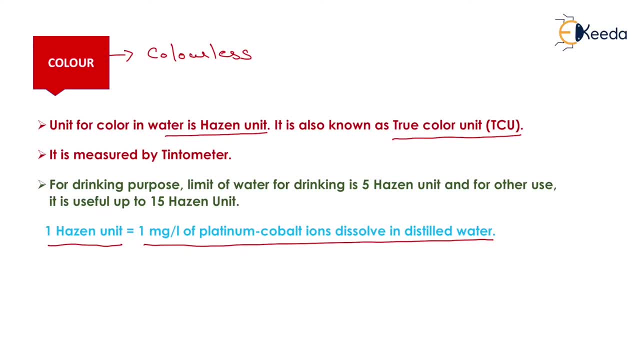 the color of that water will correspond to hazen unit or true color unit. Now, the instrument which is used for the measurement of color is tintometer. Tintometer is used for measuring the color. Now, what are the limits of color for drinking water? 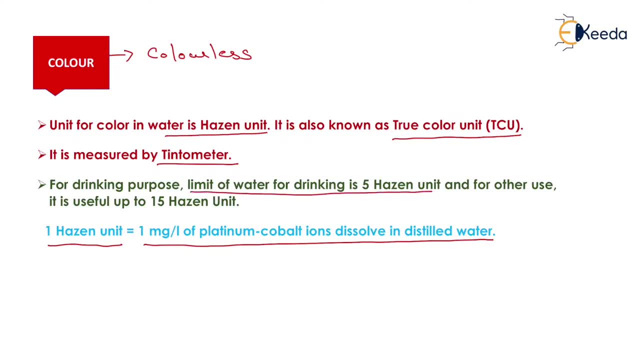 For drinking purpose. the limit of water for drinking is 5 hazen unit. It means that if the color is within the 5 hazen unit or the limit of color is within the 5 hazen unit, then that water is fit for drinking purpose. 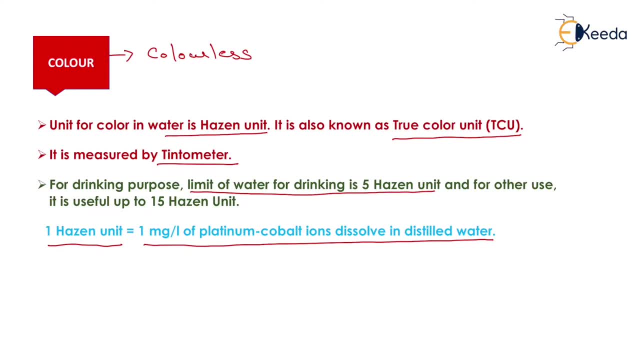 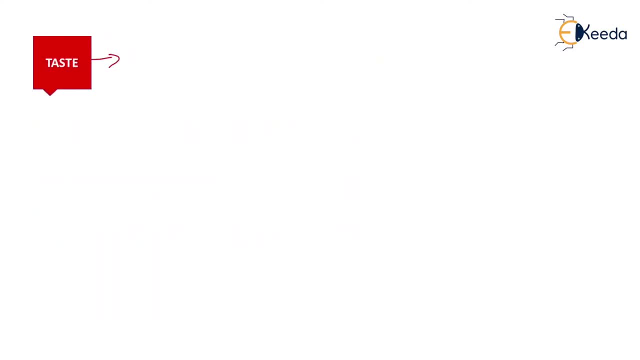 and for other purposes and or for other uses. it is useful up to 15 hazen unit. Clear. Now, moving on to the next parameter, that is, the taste. Now, the taste will depend upon the types of people which are using that water. 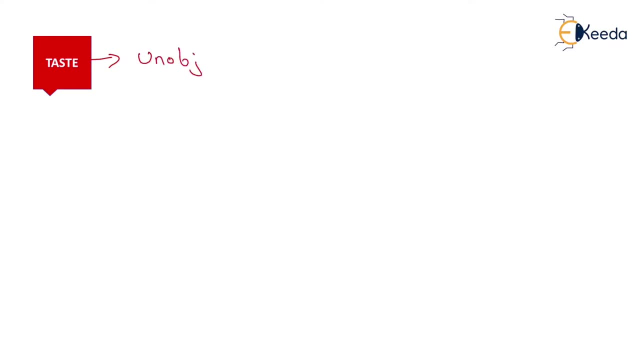 So generally it will be unobjectionable. Generally the taste will be unobjectionable because it will depend on the taste of users. Clear Now. the third one will be the odor, Generally, for all the purposes other than drinking purpose. we will take the limit of odor as unobjectionable. Okay, But for the drinking water standard generally, the value of the odor will be 1,, 2,, 3 ton. that is threshold odor number for drinking purpose. Now the question arises: what is threshold odor number? 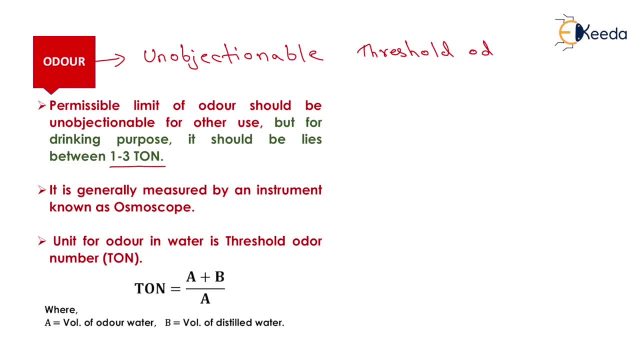